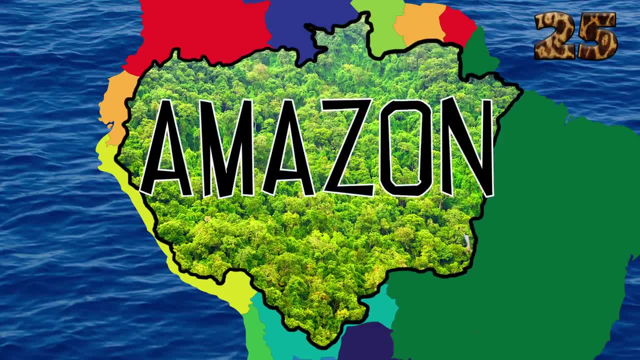 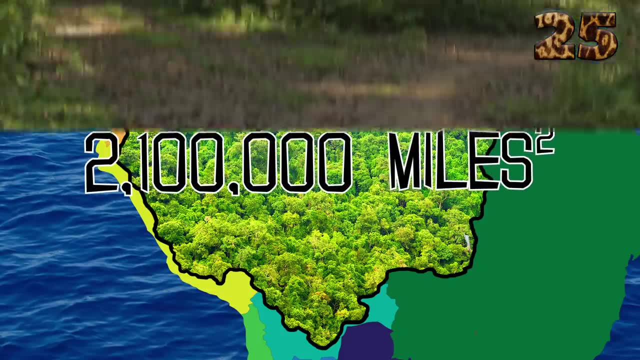 The world's largest tropical rainforest. the Amazon covers even more land than the second and third largest rainforests combined. 2,100,000 square miles of the Amazon Basin are covered in the dense tropical rainforest, so please try not to get lost. 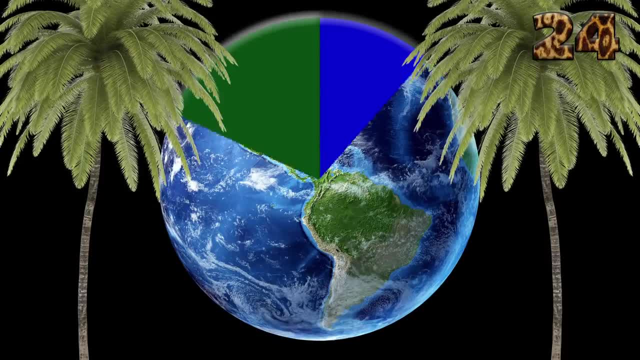 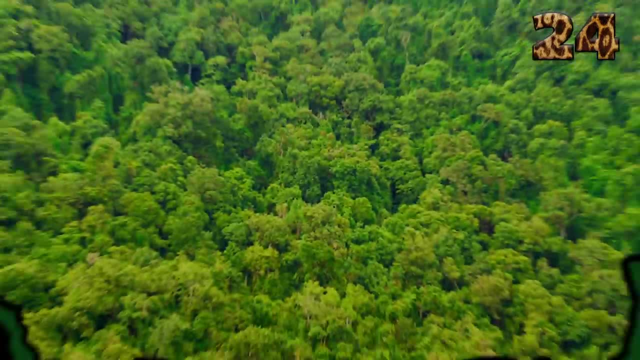 Number 24.. The Amazon Rainforest is so large, in fact, that it actually makes up more than half of the remaining rainforest land in the entire world. It's so big that it's almost the size of the continental United States. Now, that's big. 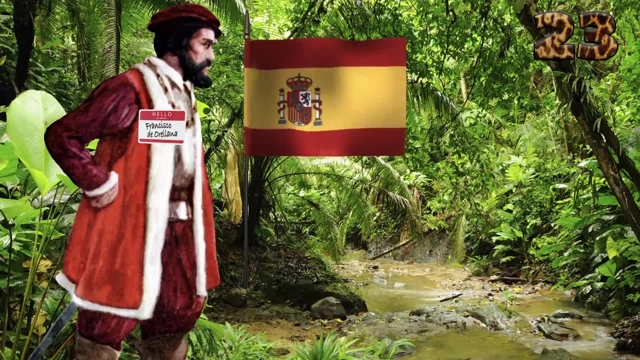 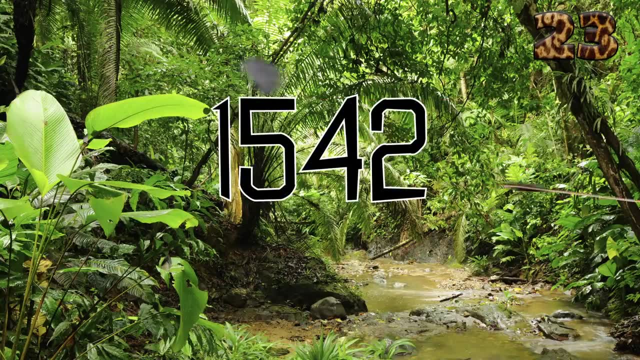 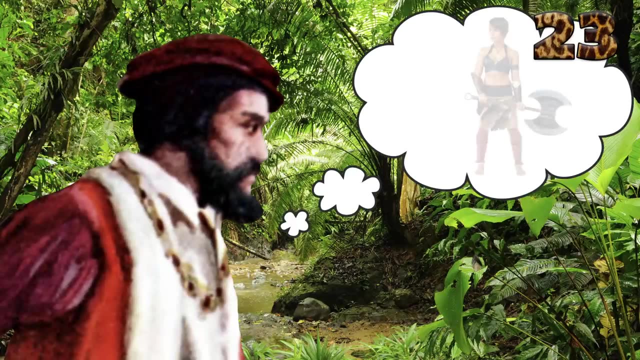 Number 23.. When a Spanish conquistador named Francisco de Oriana battled native tribes for their rainforest land in 1542, he was surprised to see women fighting alongside the men. He called the rainforest the Amazon after a group of large, fierce warrior women from Greek mythology who went by the same name. 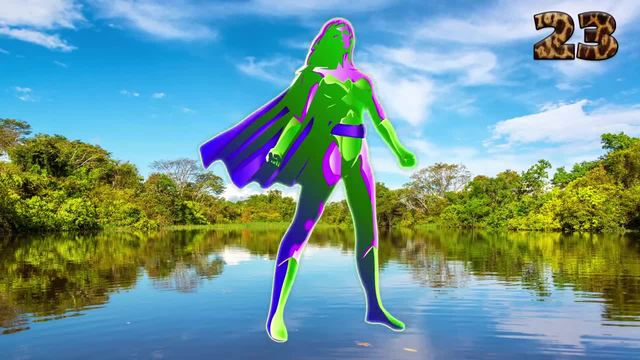 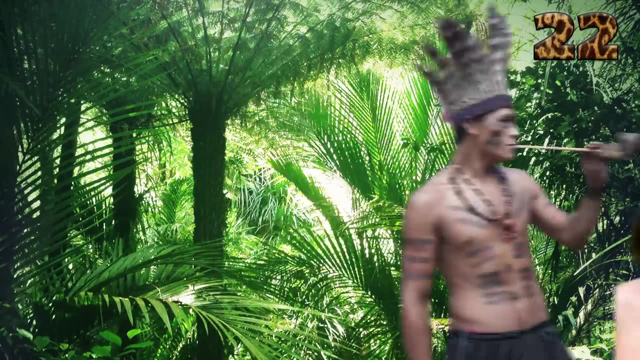 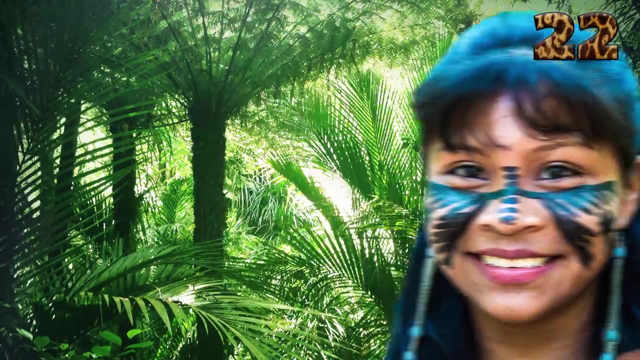 Oh, and if you happen to be looking for a cool superhero name, the forest is also known as Amazonia Nice Number 22.. There are many tribes of indigenous people who still live in the Amazon Rainforest today. Almost all of the tribes have their own culture, language, rules and territory. 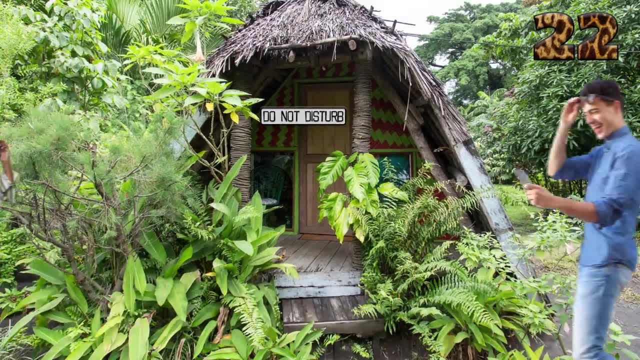 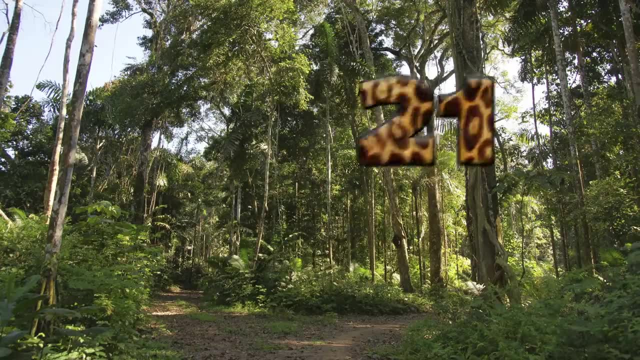 Several of the tribes have no contact with the outside world and no experience with modern technology, Which, to be honest, that probably isn't such a bad thing. Number 21. In fact, the Amazon region is actually home to more than 30 million people. 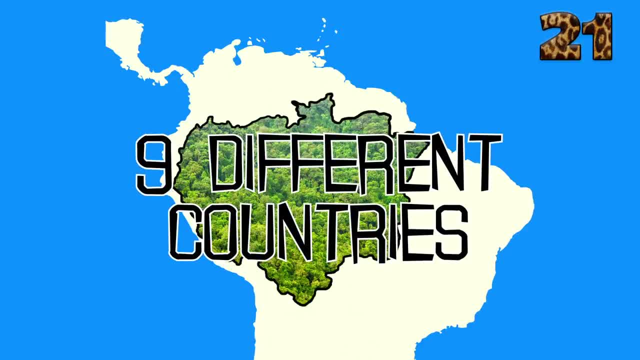 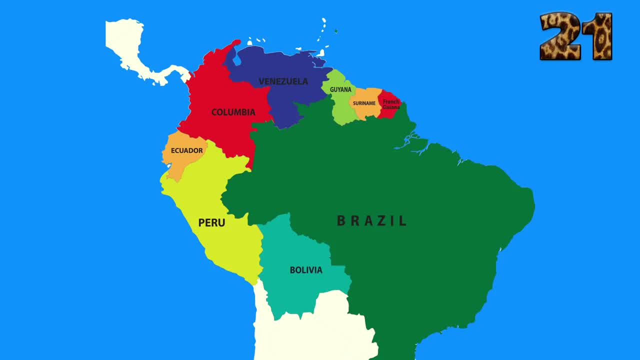 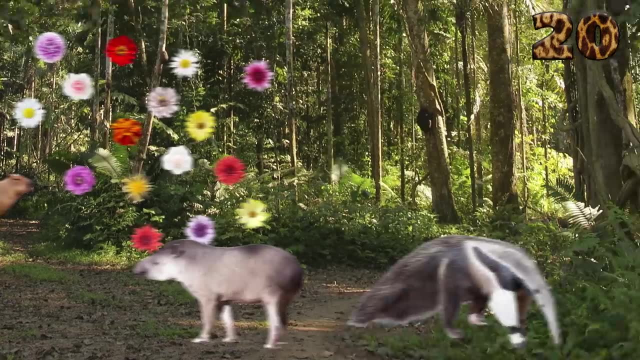 Most of the land is divided into separate territories belonging to nine different countries: Brazil, Colombia, Peru, Venezuela, Ecuador, Bolivia, Guyana, Suriname and French Guiana- Number 20.. The Amazon Rainforest's unique climate creates incredibly unique biodiversity. 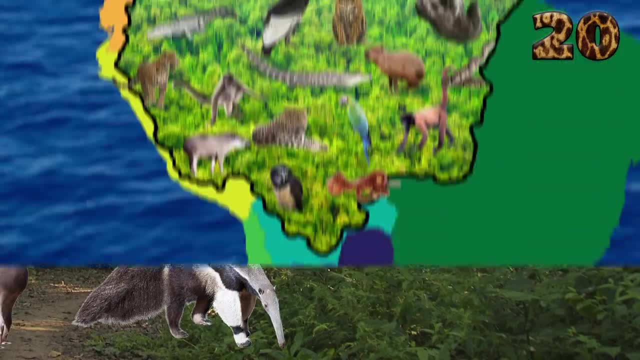 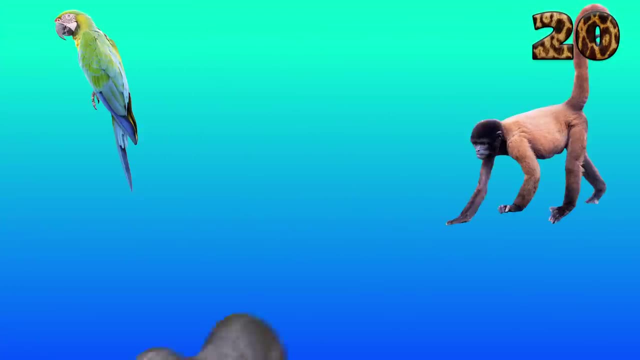 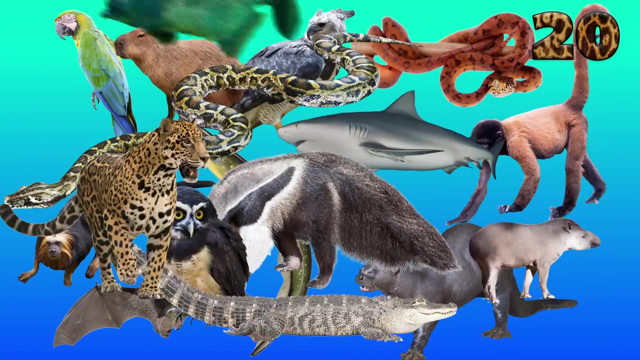 so the area's human residents have some pretty interesting neighbors. One-tenth of all known plant and animal species on the entire planet live in the Amazon Rainforest. It's the single largest collection of diverse species on Earth. In fact, the collection is actually still growing, as scientists discover even more new species every year. Whoa, Now that's awesome. That's a weird species, Number 19.. Luckily, all of these animal species are sweet, friendly and oh-so-very cuddly, right? No, Absolutely not. The Amazon Rainforest is packed with animals that want to eat you, poison you or really really just ruin your day. 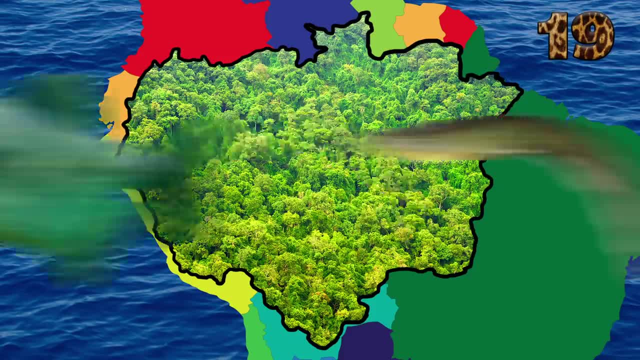 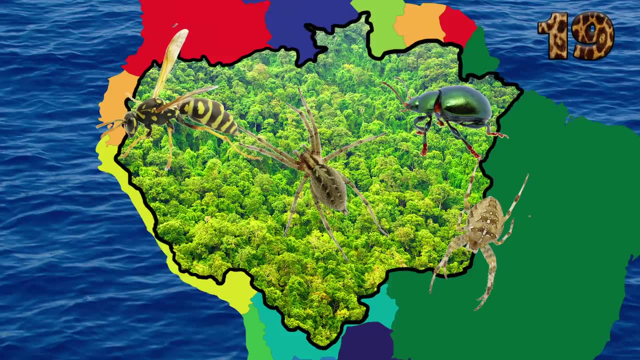 This includes anacondas, alligators, electric eels, piranhas, poison dart frogs, bull sharks, vipers, boas, spiders, bats, ants and all sorts of other deadly insects. I think I'll just stay inside for the rest of my life. 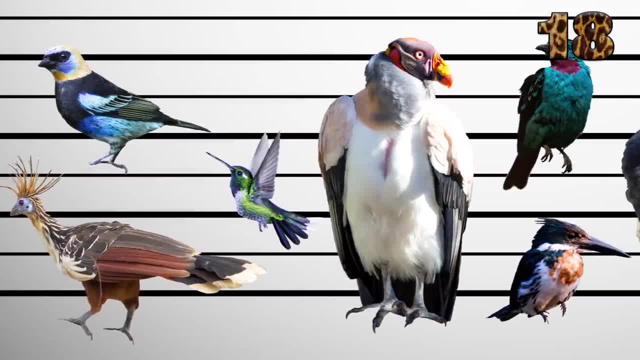 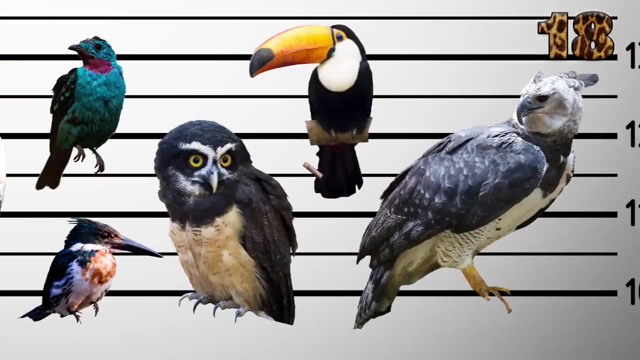 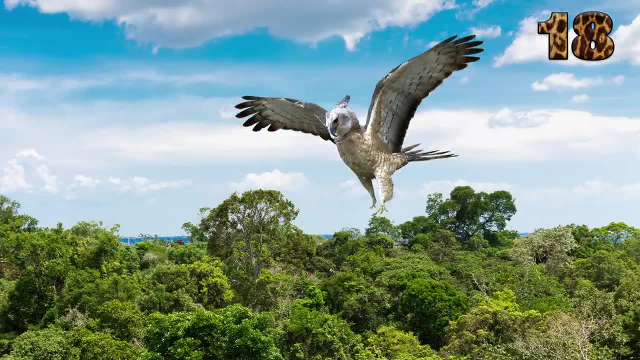 Number 18.. Even the birds in the Amazon can be deadly. The Amazon is home to one-fifth of all known bird species on Earth, and some are pretty aggressive. The harpy eagle is one of the toughest birds on the list. These large predators can grow over three feet tall with a six-foot wingspan, and they feed on mammals of all different sizes. 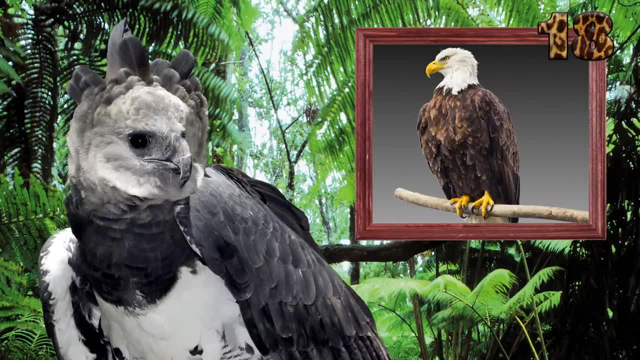 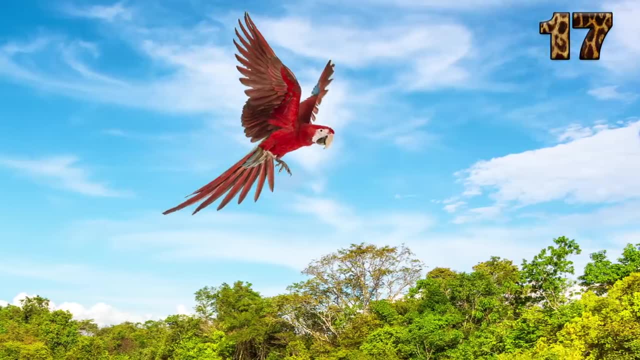 But don't confuse them with bald eagles. I hear they're pretty sensitive about that Number 17.. Macaws are also native to the Amazon Rainforest and luckily they're a bit more friendly. These birds are famous for their beautiful feathers. 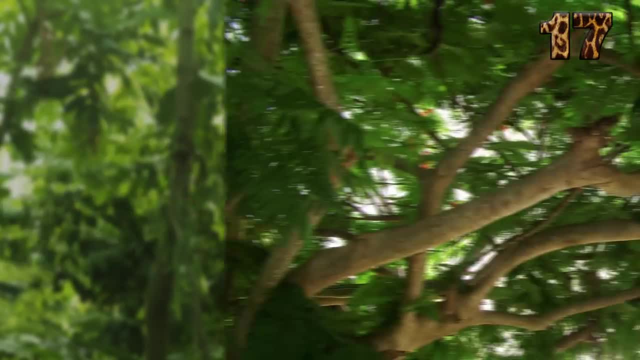 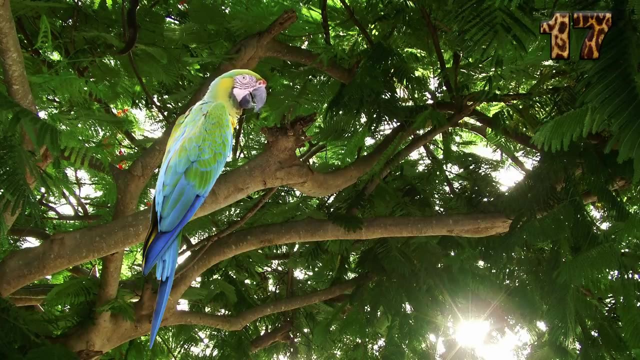 Their tongues also have a thick bone that helps them crack nut shells. They're also remarkably good at mimicking human speech. Hey, Hey, That's good, That's good. Okay, Okay, Stop copying me, Stop copying me. Seriously, Seriously, Come on, Come on. 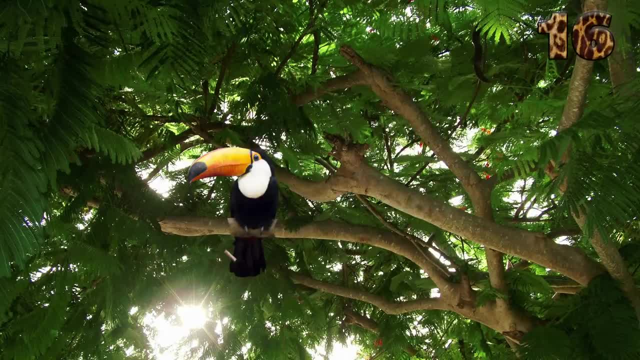 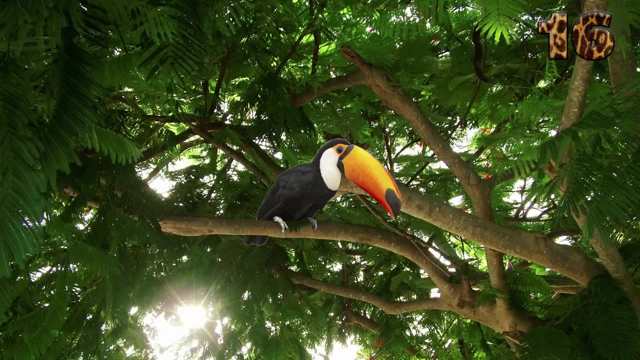 Thumb bird says what Thumb bird says what Number 16.. The toucan has become a symbol for the Amazon Rainforest. even though they mostly stay hidden high up in the canopy layer, Their brightly colored bills can be over half the length of their bodies. 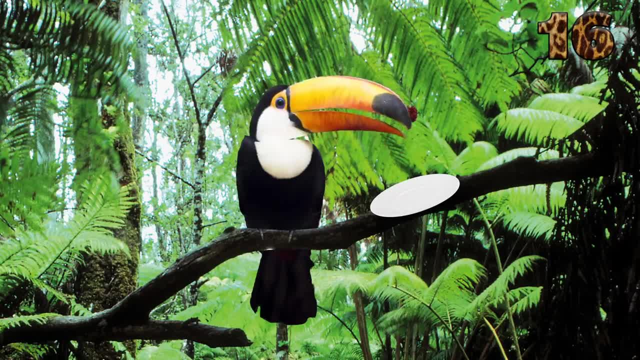 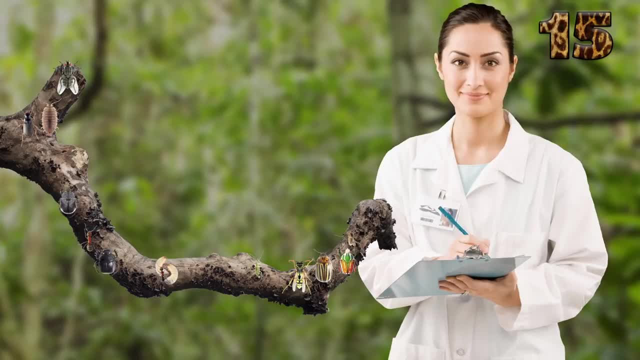 But don't worry, They're very light and easy to maneuver. These bills help the toucan reach fruit from high branches and bugs that are burrowed deep inside of trees- Number 15. Speaking of bugs, there are so many insects in the Amazon Rainforest. 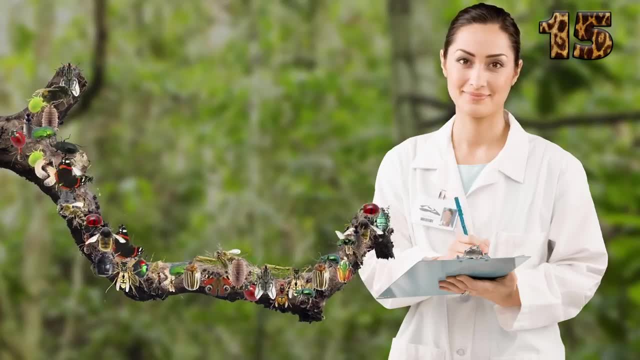 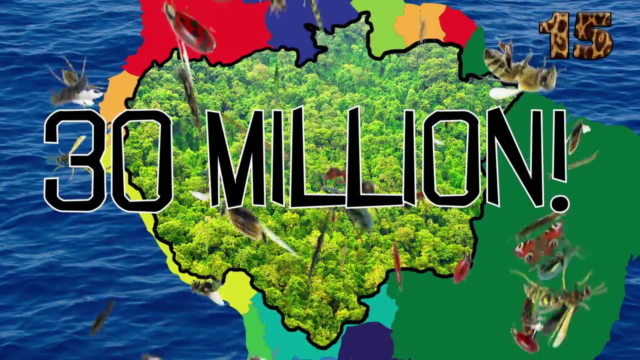 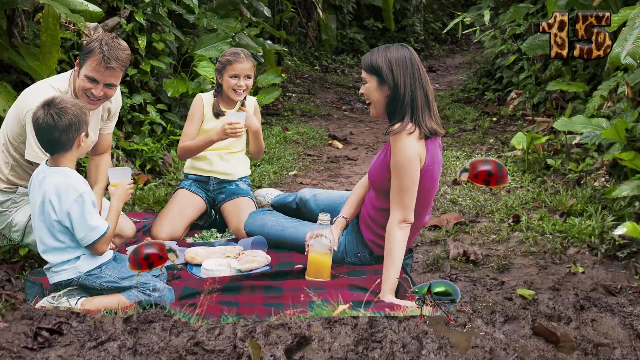 that it's impossible to get an accurate count of how many different species there are Right now. the best estimate of experts is about 30 million. One acre of forest may have almost 70,000 different species of insects. So, yeah, this might not be the best spot for a picnic. 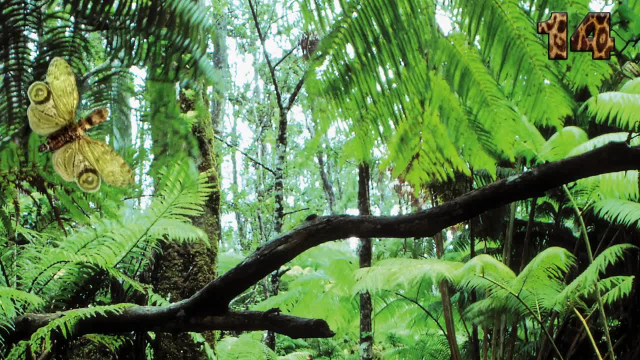 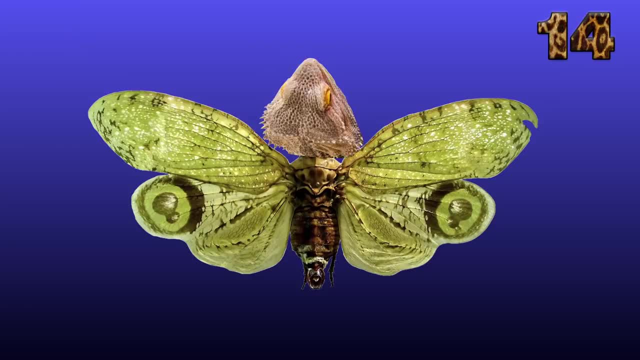 Number 14.. One of the weirdest looking insects from the Amazon Rainforest is the peanut-headed lanternfly. The unique shape of their head is supposed to mimic the head of a lizard or a snake to scare off predators. If that fails, they have big fake eyeballs on their wings. 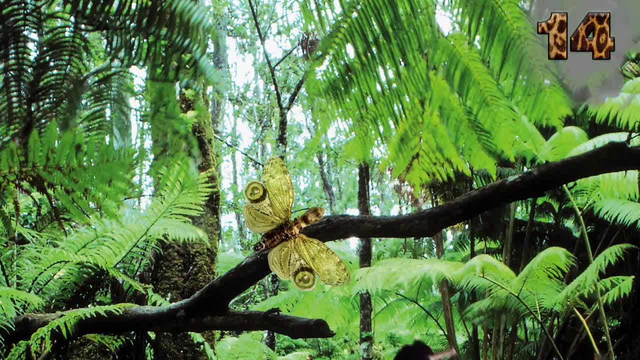 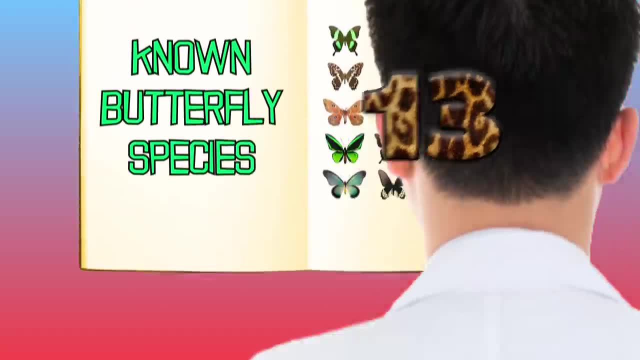 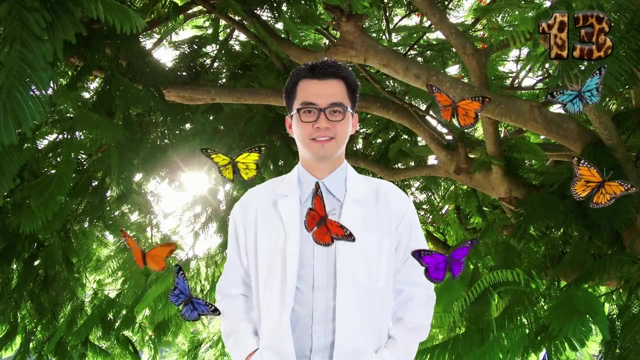 When threatened, they also release a foul-smelling substance that helps them escape. At least, that's their excuse Number 13. There are about 20,000 known species of butterflies in the world, and a whopping 7,000 of those species are found in the Amazon. 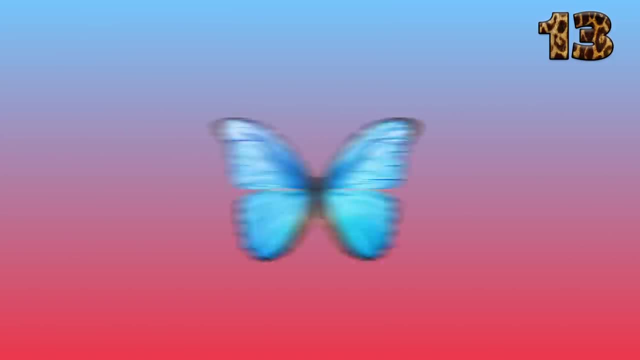 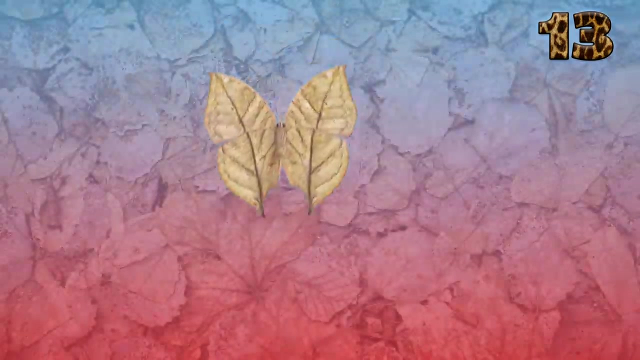 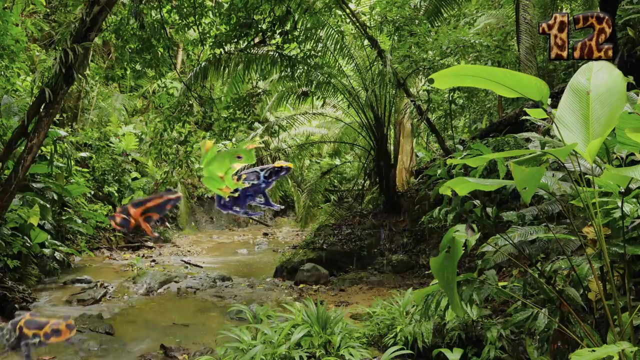 Some of them are truly beautiful- hues of blue, red, black, green, yellow and, well, every color there is- And others are masters of disguise, mimicking the patterns of fallout. Hey, where'd he go, Number 12.. The Amazon is also home to tons of different species of frogs and toads. 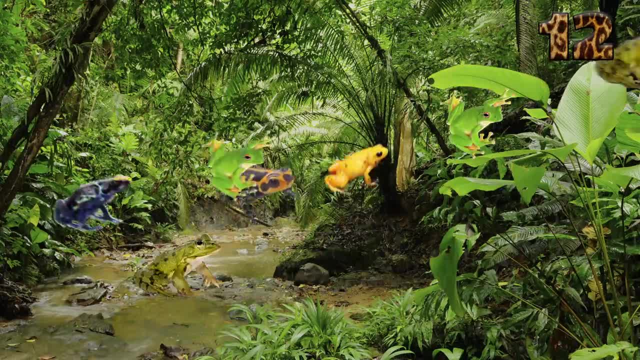 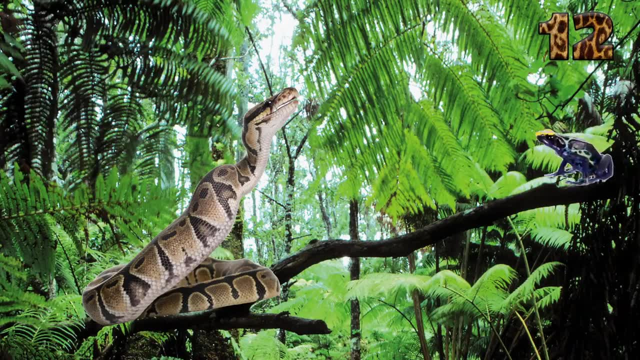 The air is so humid and it rains so often in the Amazon that these amphibians don't have to live by bodies of water like in other parts of the world. Instead, they'll climb trees to explore and escape predators. But actually a lot of the species don't really have to worry about predators at all, because they're so poisonous. 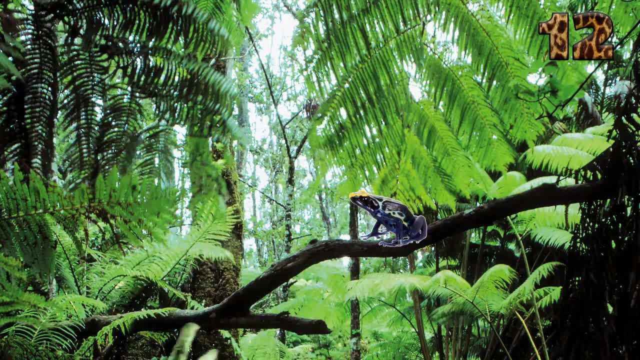 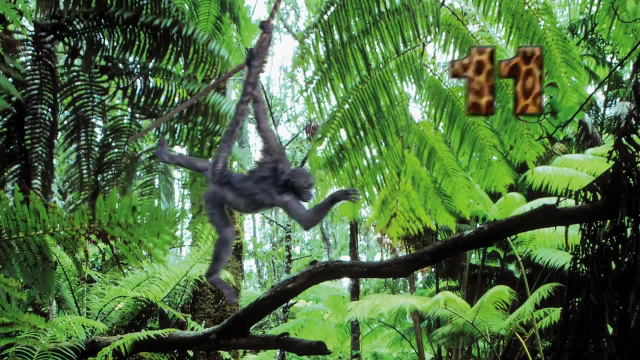 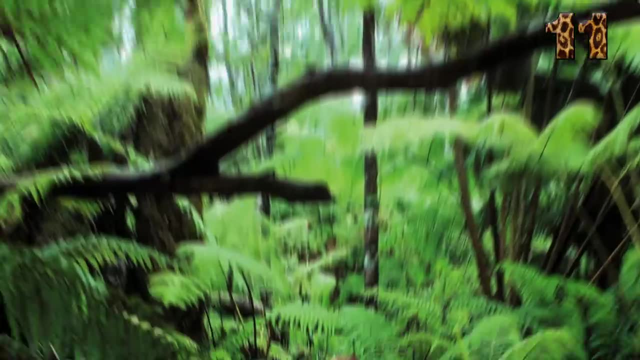 Take the brightly colored poison dog, The dart frog we talked about in our deadliest animals episode, for example. They may look cute, but they're stone cold killers Number 11.. The Amazon is also chock full of monkeys. There are many different species that range in size and level of intelligence. 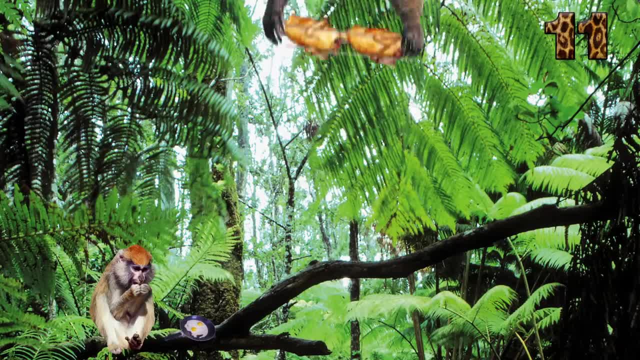 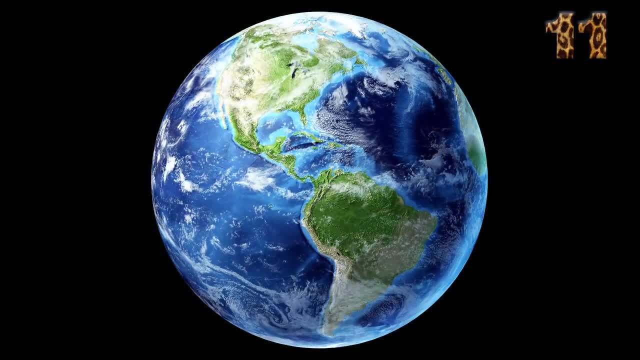 Most of them eat fruit and nuts, but some eat bird's eggs and even birds themselves. The howler monkeys that live in the Amazon rainforest are the loudest land animals in the entire world. Their territorial call can be heard from over three miles away. 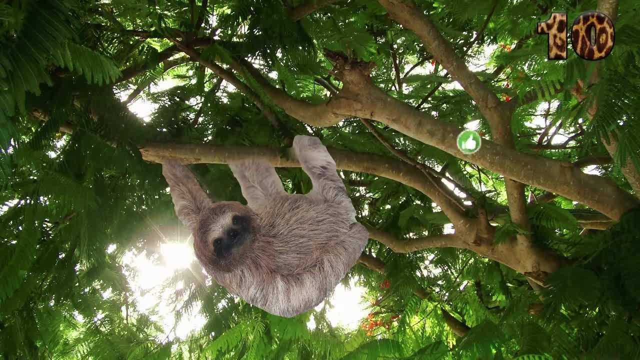 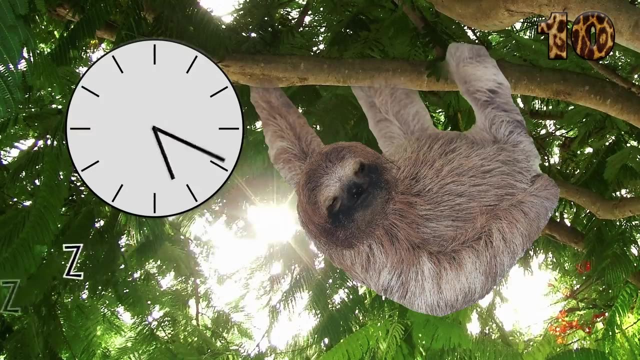 Number 10.. Three-toed sloths are some of the most popular animals that come from the Amazon rainforest. They're super cute, but also super lazy- So lazy, in fact, that algae actually grows on their fur. They sleep up to 20 hours a day, and even when they're awake they don't do much except hang around in trees. 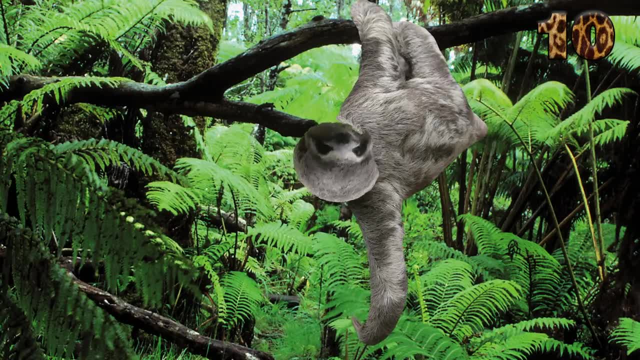 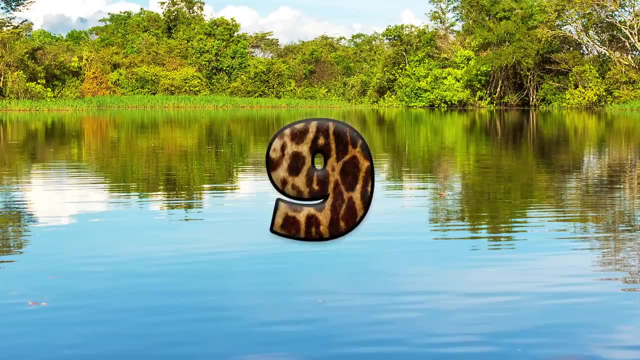 They have a few hidden talents though. They can rotate their heads almost all the way around, and when they fall into the water they're actually pretty strong swimmers. Go for the gold Number 9.. The Amazon basin is home to the majestic pink dolphin. 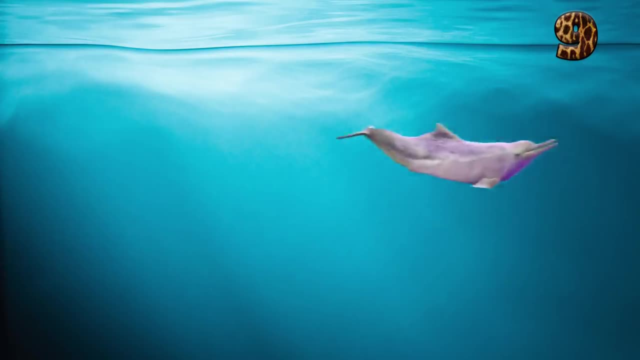 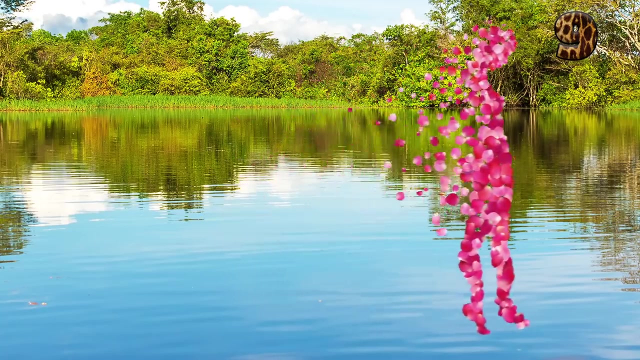 These large freshwater dolphins can grow over eight feet long and usually swim around alone. In Amazonian folklore, these dolphins are said to be shapeshifters. It's considered bad luck to kill a pink dolphin, and if you look into a dolphin's eyes, you may have lifelong nightmares. 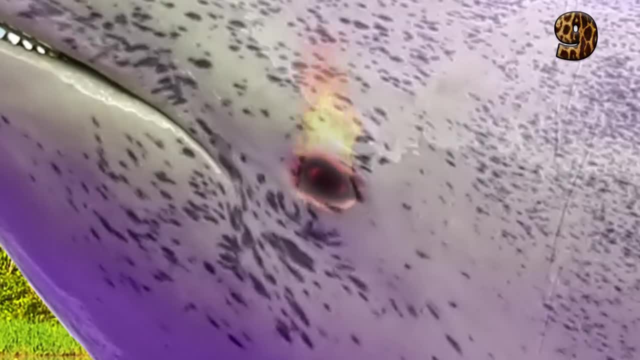 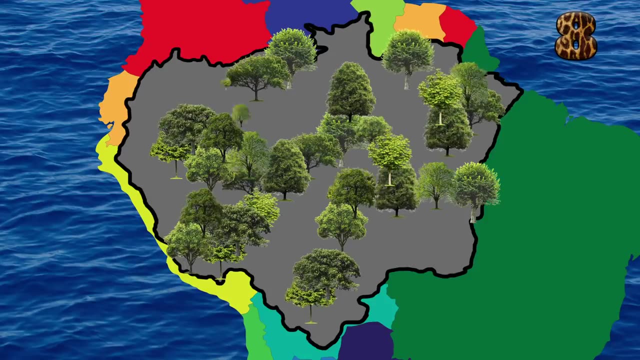 I mean, if you believe that sort of thing, I'll be right back. I'm gonna go buy a nightlight Number 8.. There are a lot of trees in the rainforest, Like a lot of trees, Like a lot, a lot. 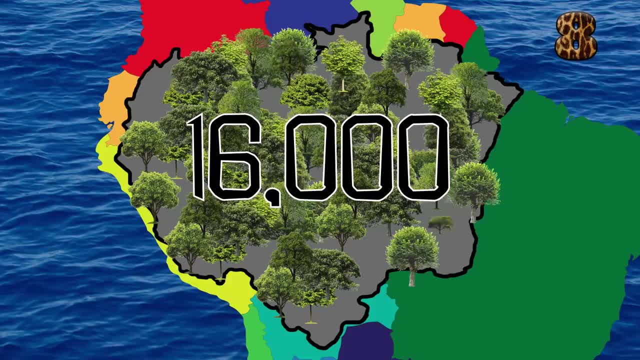 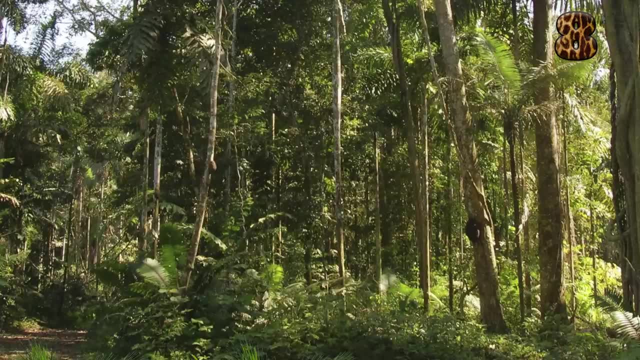 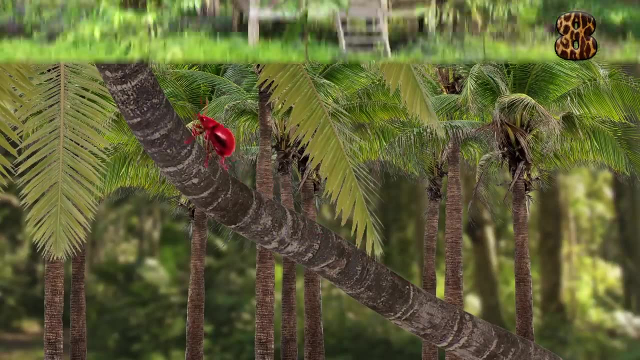 There are almost 16,000 different species of trees in the Amazon and they combine to create a dense forest of about 390 billion trees. That's so many trees. These trees create natural materials and provide homes for most of the insects, birds and animals of the Amazon. 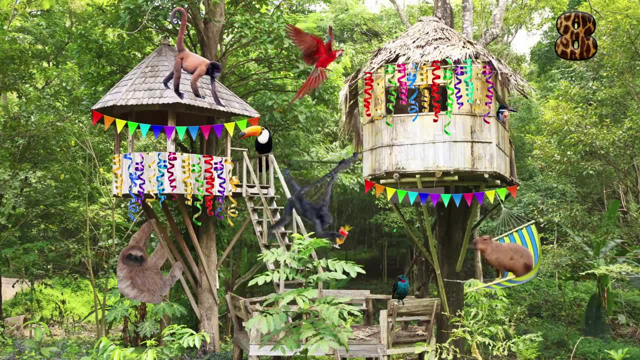 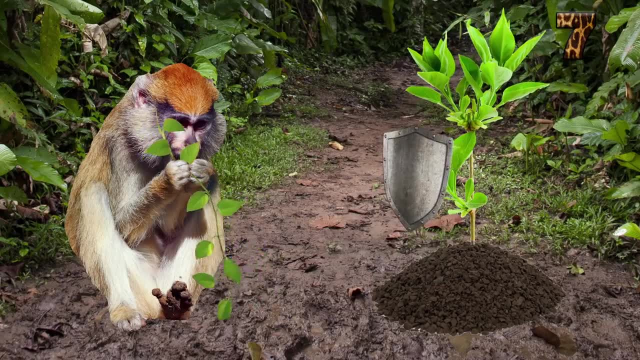 Well, that's not really what I meant about living in trees, but uh, who cares? This is awesome, Number 7. Many rainforest plants have developed special natural defense systems so that animals won't eat them. Some plants have hard outer layers which make them hard for animals to break down and eat. 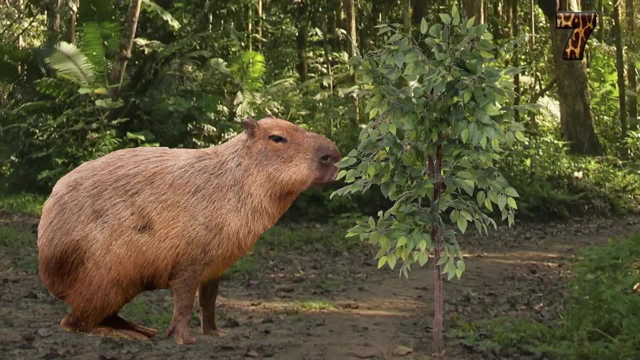 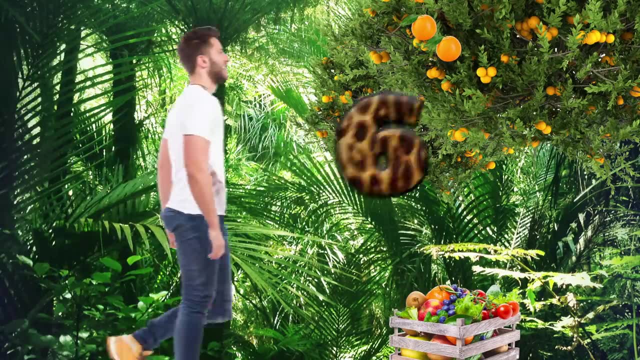 Some have become tasteless or super bitter. Some of the plants have even developed poison to protect themselves. I'm not sure what that one does, but I'd steer clear Number 6.. The Amazon rainforest is home to over 3,000 different kinds of fruit. 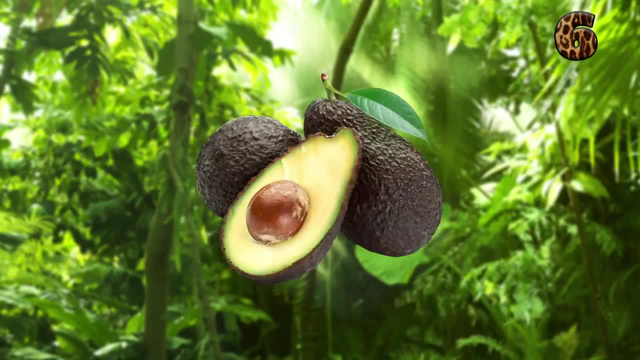 Only around 200 are commonly used in the Western world, like avocados, coconuts, figs, oranges, lemons, grapefruit, bananas, guavas, pineapples, mangoes and tomatoes. You get the picture. 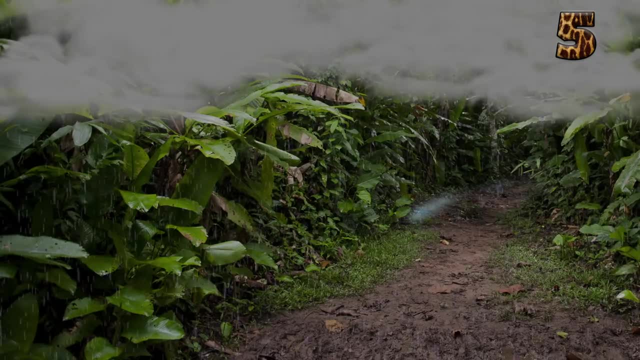 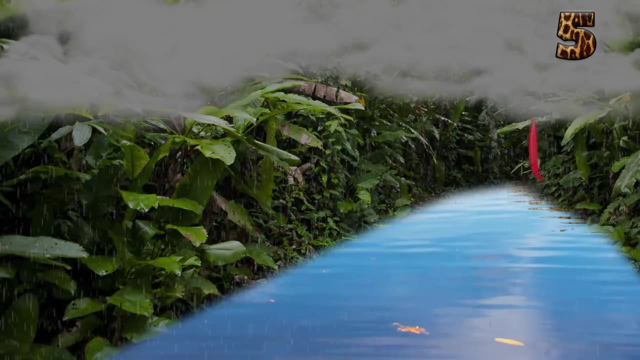 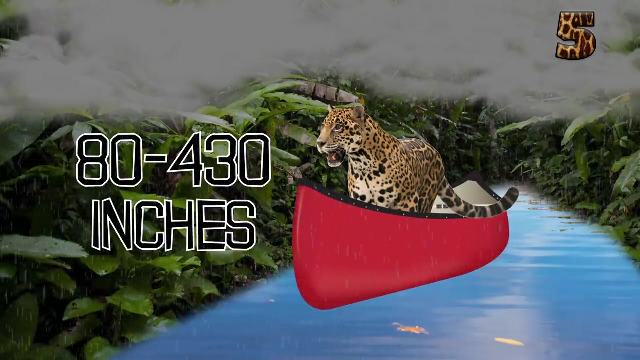 Number 5.. Trust me, the Amazon rainforest isn't called a rainforest for no good reason. The Amazon creates almost 50% of its own precipitation because of the dense trees that keep the moisture in. It can see anywhere between 80 and 430 inches of rain throughout the year. But, that being said, it does still see long dry periods that can cause droughts and do damage to some of the wildlife. Number 4. The canopy layer, aka the layer where the leaves and branches of dense trees interweave. 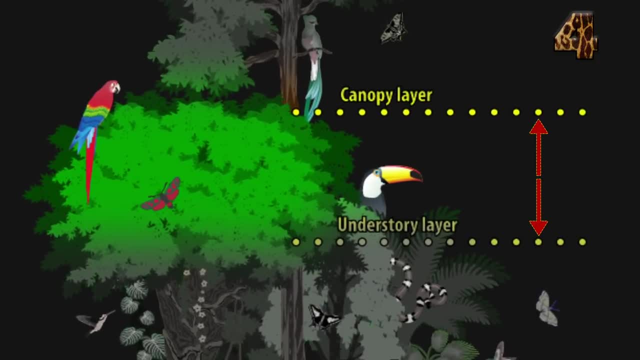 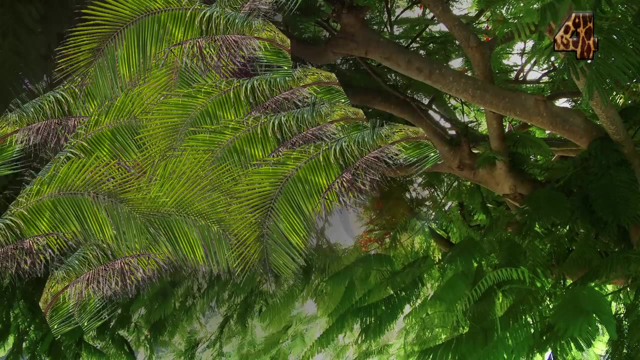 can be composed of almost 100 feet of vegetation. This covering of leaves is so thick that it leaves a lot of the forest floor so dark that most plants can't grow on the ground. Sometimes it can take 10 full minutes for rain to pass through the canopy layer. 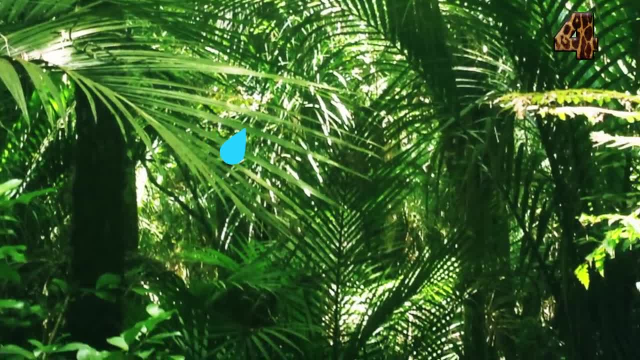 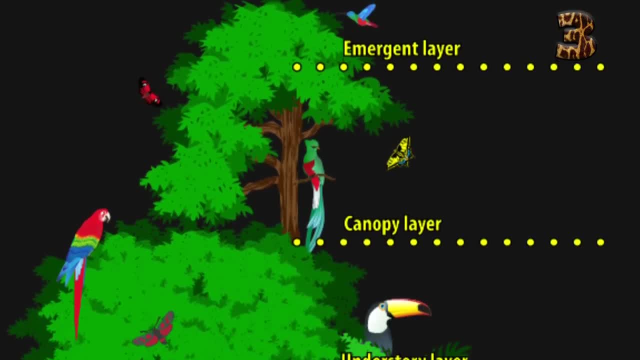 Alright, any second now Come on. Ah, forget it. Number 3.. Let's break down the layers of the Amazon. There's four main layers: The emergent layer, the canopy layer, the understory layer and the forest floor. 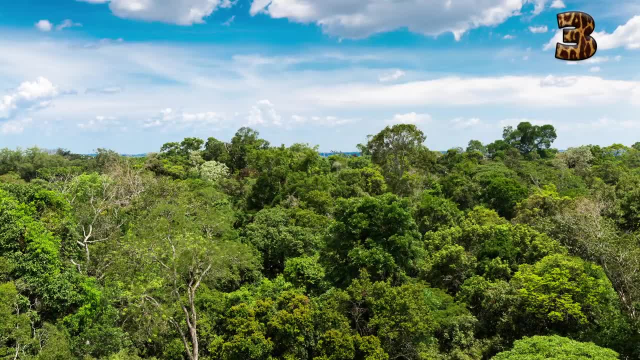 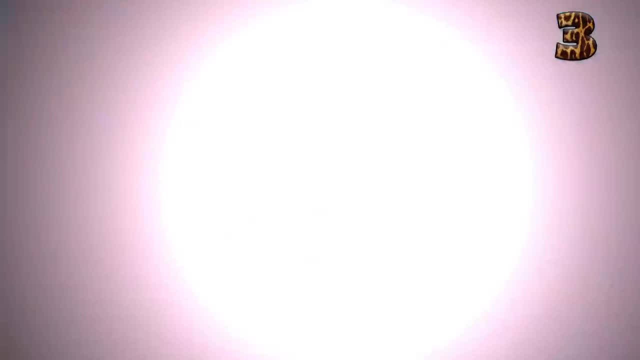 The emergent layer is the highest level of the rainforest. The giant trees have huge mushroom-shaped crowns that cover everything below. Since it's the layer that touches the sky, it gets by far the most sunlight, but also endures high temperatures, low humidity and strong winds. 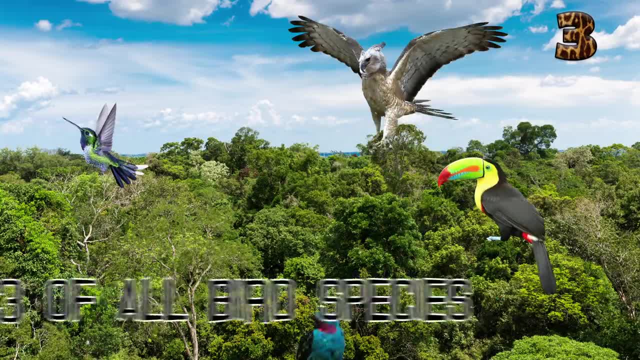 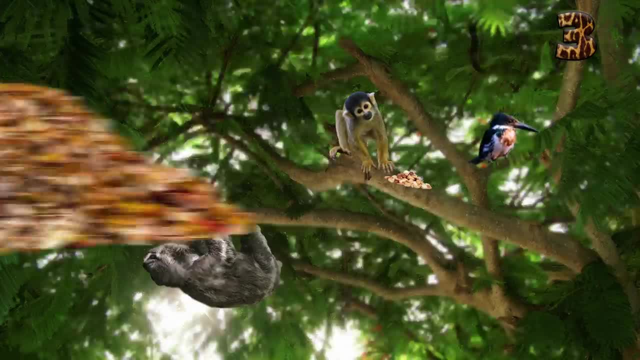 It's also the world's biggest natural aviate. Nearly one-third of the bird species on Earth live there. The canopy layer is found directly beneath the emergent layer. The branches are covered with leaves, plants, vines and food for small animals. 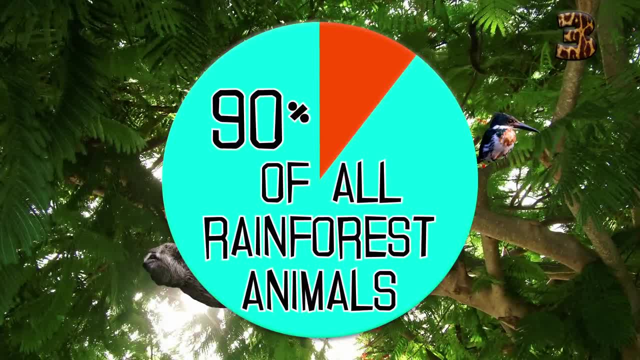 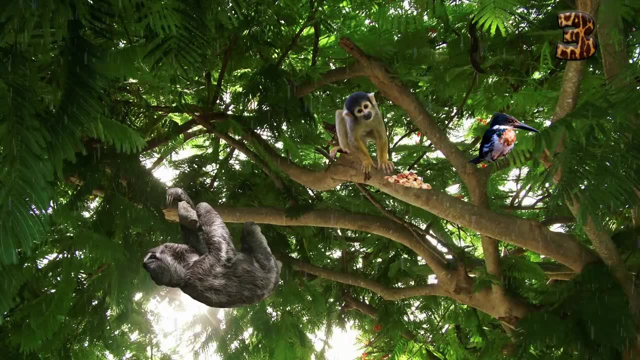 The canopy is home to 90% of all animals found in the rainforest. The canopy gets the second most sunlight of all the layers and is protected from the sun's UV rays. This layer also retains moisture and creates a natural umbrella in the tropical rainy season. 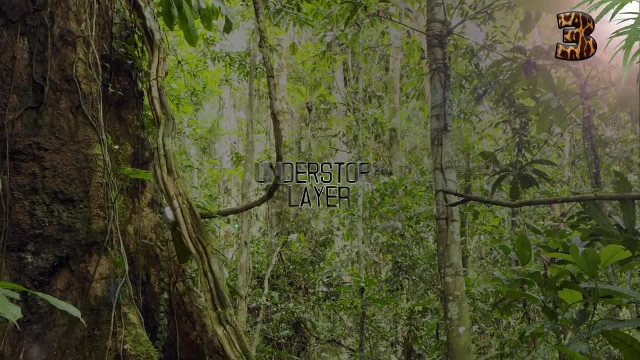 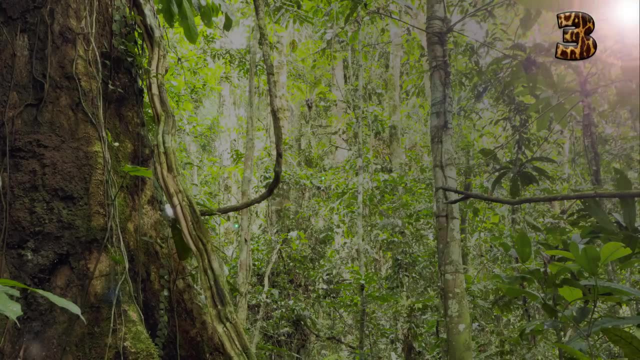 The understory layer receives only 2-15% of the sunlight that falls on the canopy layer above. Because of this, the understory is a dark, almost impenetrable layer full of vines, shrubs and trees. This layer creates natural camouflage for the animals that live there. 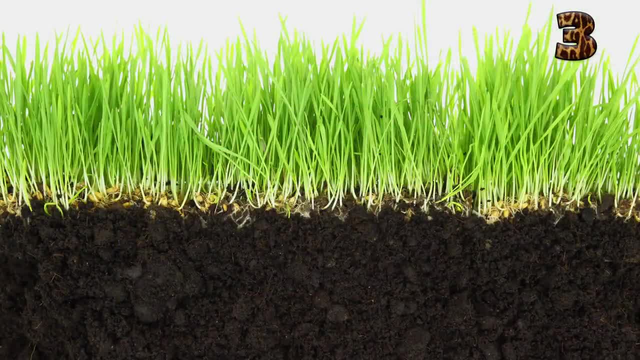 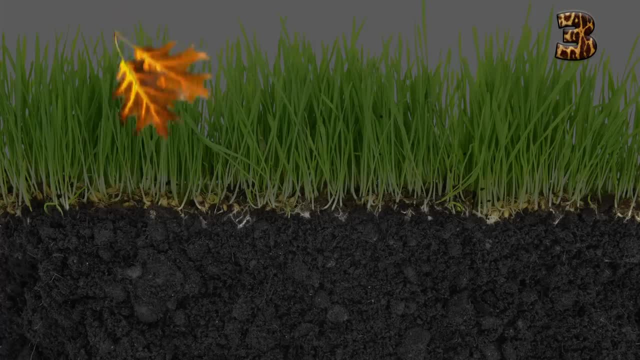 The bottom layer is the forest floor. Only 2% of the sunlight makes it through the other three layers, so it's extremely dark year-round. The quality of soil is very poor, so the floor is mostly a thin layer of fallen leaves, seeds, fruits and branches that decompose quickly due to the warmth and moisture. 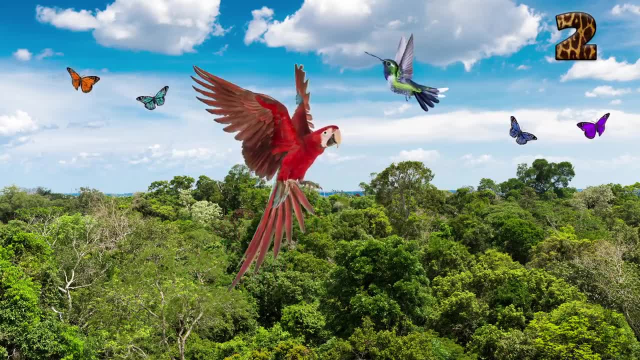 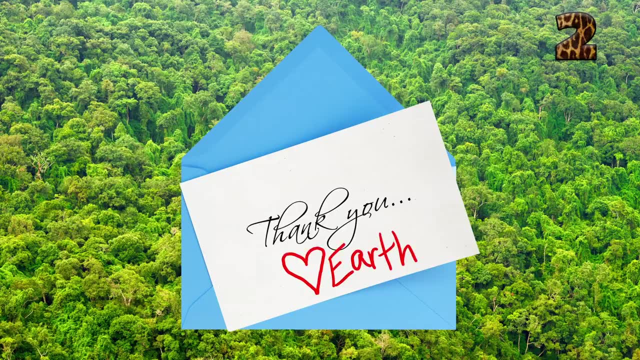 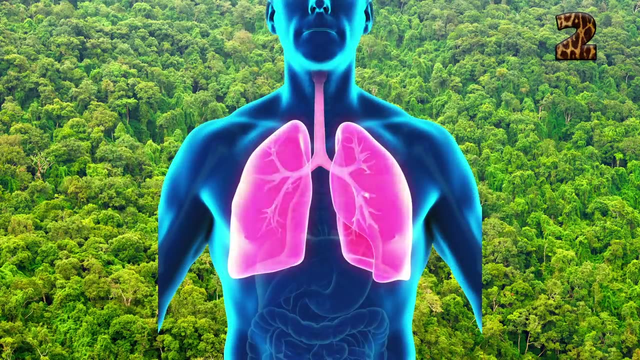 Number 2: Take a deep breath of fresh air. Who wasn't that peaceful? You can thank the Amazon rainforest for that moment of serenity. The trees in the Amazon produce more than 20% of the world's oxygen. The rainforest is affectionately known as the lungs of the world. But if you're taking a deep breath directly inside the rainforest, you might want to be careful, Eww. And finally, our number one fact is by far the most important one too: The Amazon rainforest has fallen victim to deforestation. 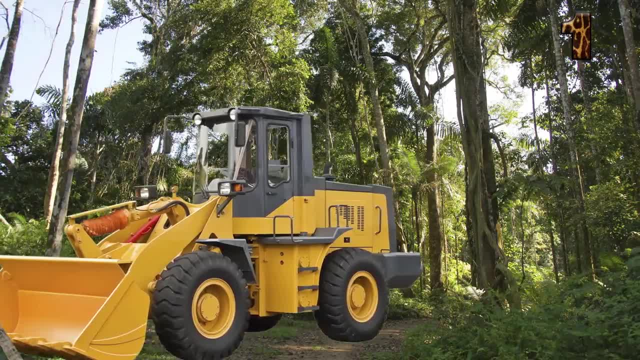 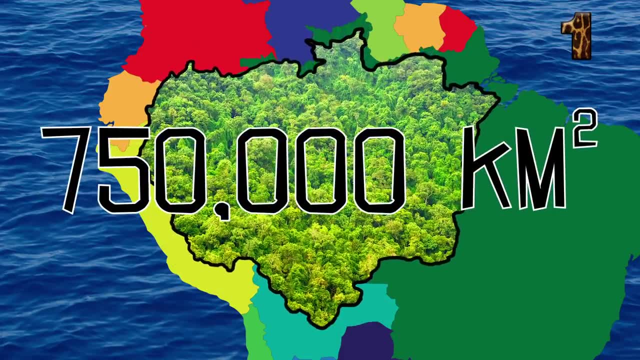 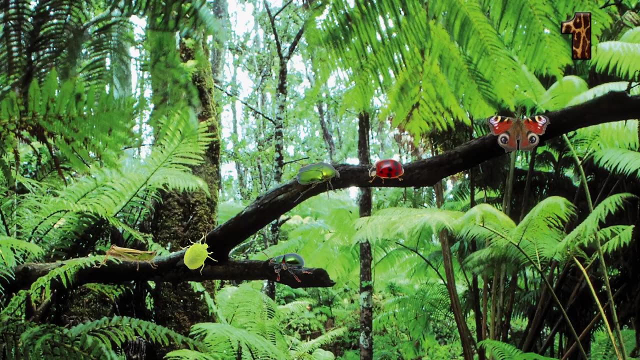 That means that as we chop down trees for materials and space for crops, we do severe damage to the Amazon's fragile ecosystem. Over 750,000 square kilometers of the forest have already been lost. Many species of insects have been entirely wiped out before they could even be studied. 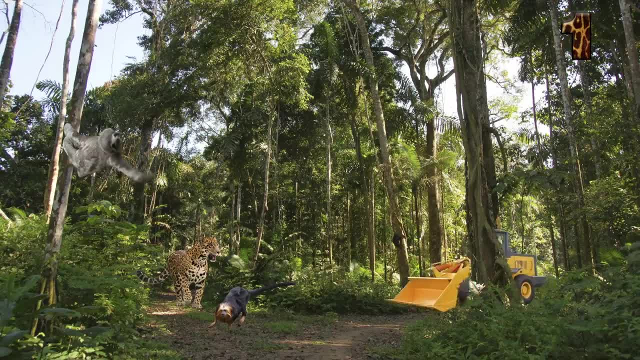 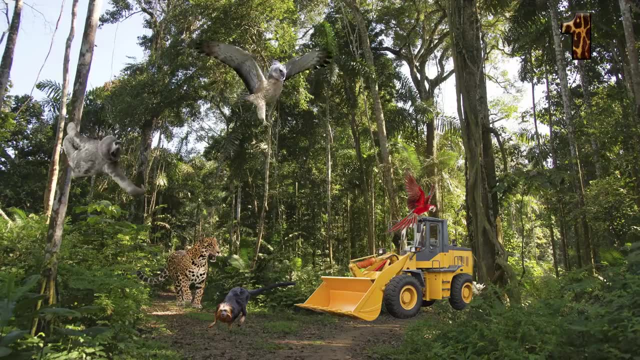 And that's all really sad. but there is a bit of good news: We're starting to make some progress toward preserving the rainforest and the wildlife within it, as more and more people choose to fight to protect it. The Amazon is a unique and irreplaceable piece of our planet.